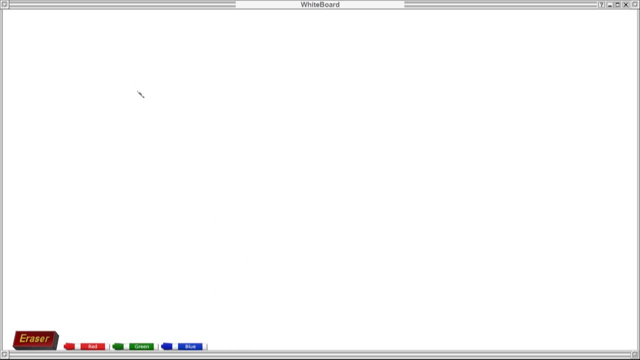 So today, what I'm going to be talking about is electromagnetic induction. Okay, This is an A here. I'm still not used to doing this. Okay, Okay, Electromagnetic induction, And what this is is pretty much the AC: electrical current is induced through an electromagnetic field. 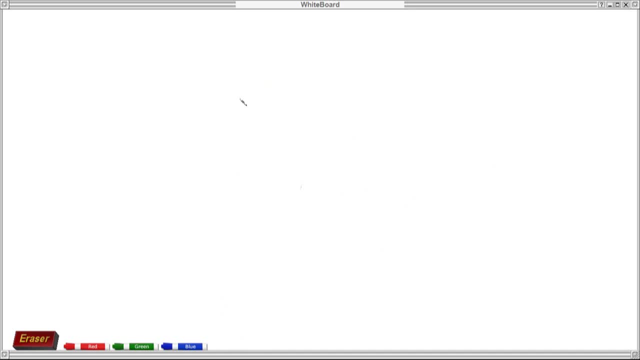 Now, originally, when I was growing up, I used to do this. I used to do this kind of thing, This kind of thing, But today I'm going to be doing a special tutorial about this. Okay, Electromagnetic induction And what this is is pretty much the A here. I'm still not used to doing this. Okay, When people started using electricity it was just well. batteries weren't really that good back then. They weren't really as good as they are now, considering how much nanotechnology that there is to improve quality of batteries or even create new types of batteries. 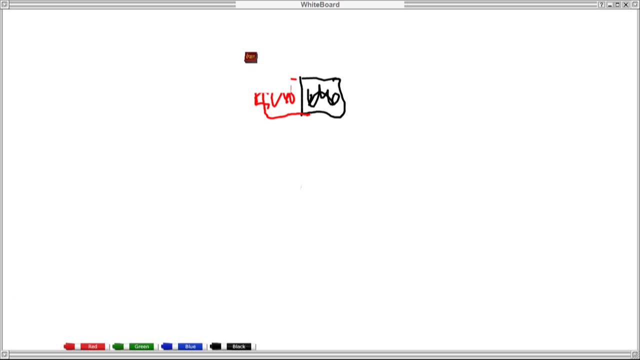 Or even any of these lithium ion batteries that there were, And basically all it was is it was just a lot of. it was produced to a variety of different apparatuses. Some were, some were created electrostatically, and it's just a gathering of electrostatic and all. 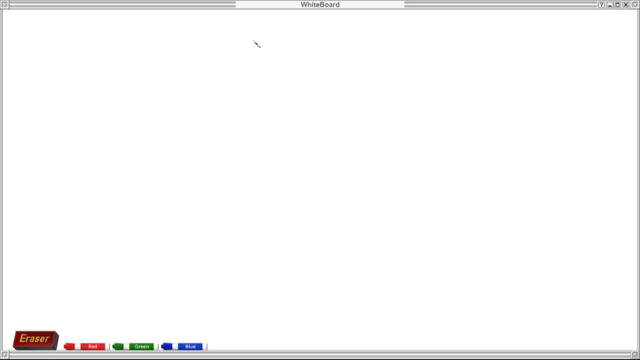 And they didn't have any induction motors. They didn't AC, in reality didn't exist at all. It wasn't until later on, when Nikola Tesla came around, where we're pretty much AC, DC, current and all these other technologies started To be implemented. The guy was a genius and all But anyway. so basically a lot of a lot of the telecommunication technology is based on electromagnetic induction. 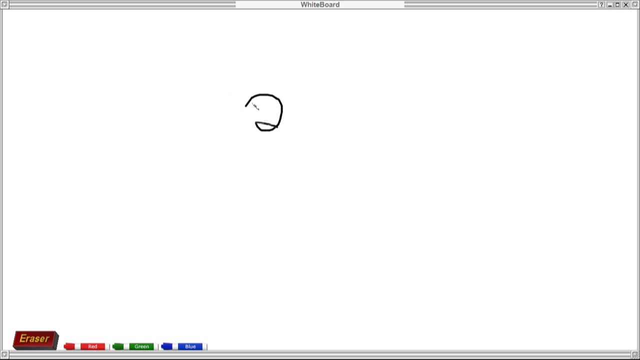 And basically what it is is is just transformers. Okay, It's just an electrical transform transformer. There's. the most common type of electrical transformer is the iron core, And usually what you have is your, you have your turn ratio. Okay, So let's say, for example, you want to put, you want to put, put a certain amount of voltage. 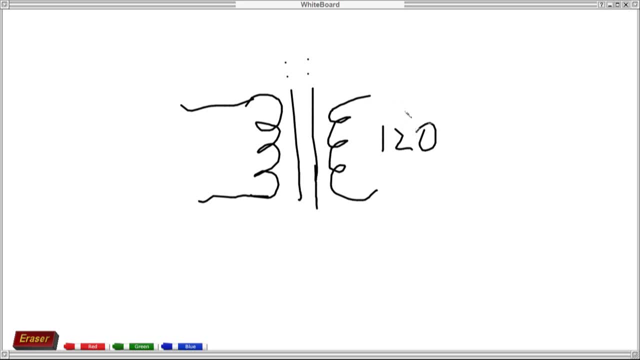 You get your typical 120 volts. Okay, So the formula for this is basically your, your primary B source divided by your secondary B source is equal to your turn ratio, which is your primary B source. And the way this works is that if you, let's say, you want to get the amount of, let's say, you want to get the amount of primary B tissue, you, you want, want this apparatus to to have, and you want to get, you want to get the amount of primary B tissue. 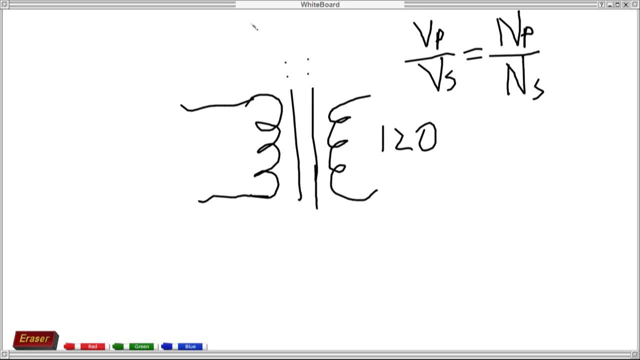 Okay, How much? um, basically, you want to know how much turns how much power and how much electrical power you need to feed into it, How much electric, uh, uh, electric electrical voltage you want to get get through here. 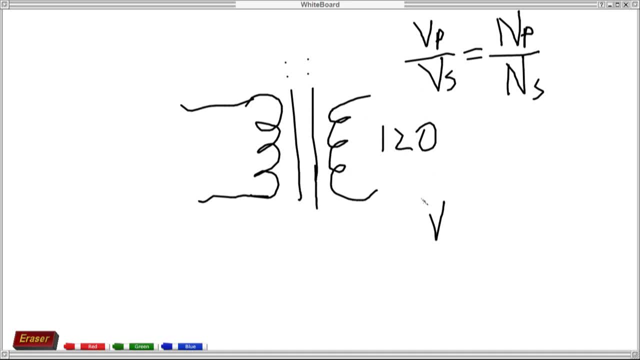 You basically have to uh do this. Your primary voltage is equal to your uh primary uh turn rate. uh turn ratio divided by Your set uh. your secondary turn ratio times your uh secondary voltage. Okay, 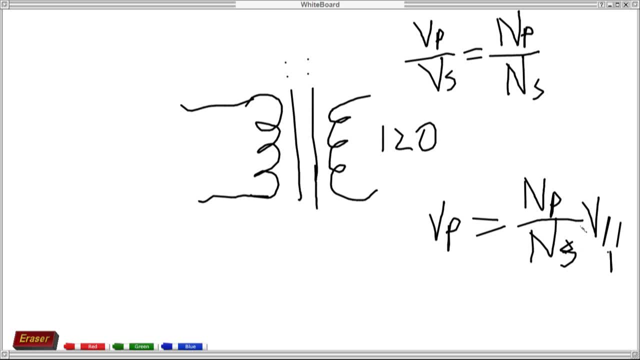 Hold on, Let me get this. Okay, I can't, I can't, I can't draw that well on the edge or anything for some reason, But uh, anyway, Um, y'all kind of get the, y'all kind of get the idea of this. 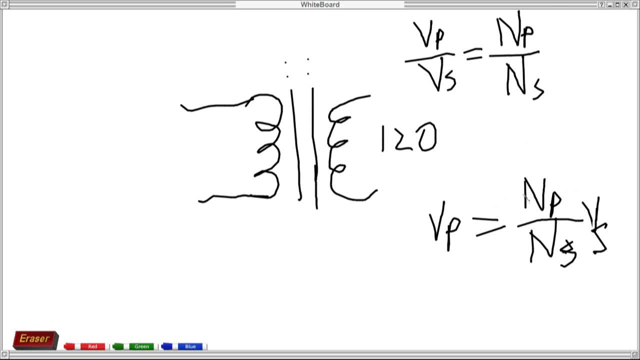 Okay. So anyway, your um, your um, B, primary, Okay. And let's say, for example, this is um, this is a 10 to 1 ratio. So what that means is: uh, you have to look what we uh, what we have here. 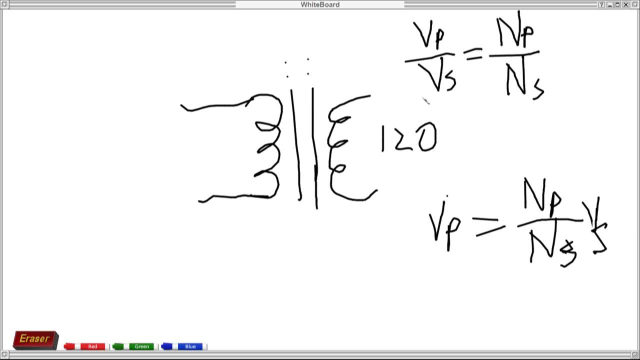 And what we have here is 120 volts AC. Okay So, um, we don't know our B primary yet. Okay So, equal And um, the primary, um, the primary number of turns is going to be 10.. 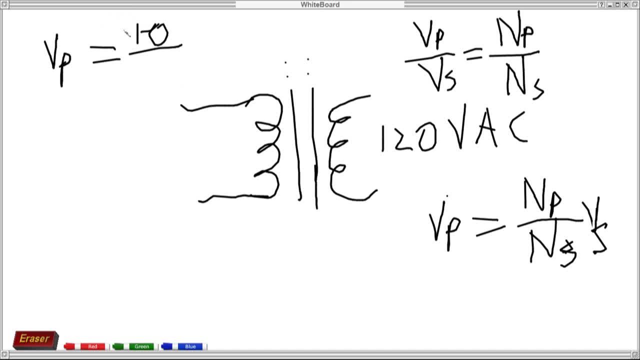 Uh, it's 10.. And your secondary is going to be uh 1.. Okay, So what this means is not: it doesn't mean that necessarily mean that you have 10 turns per uh, 10 turns here and 1 turn here. 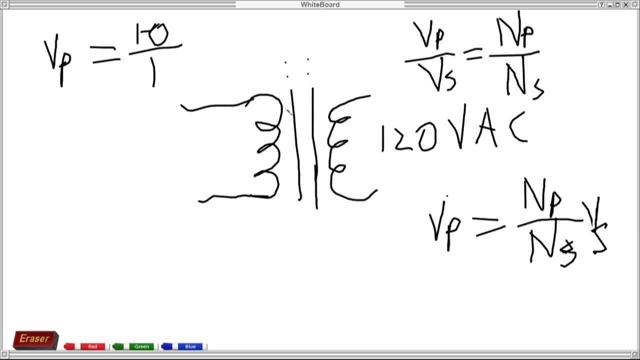 Even though you could do that, it wouldn't be effective because it's likely to burn out depending on, of course, depending on the thickness of the wire, the length and all that, And, um, the thickness of the core here. So this is what you are going to do, uh, inducing through and on. 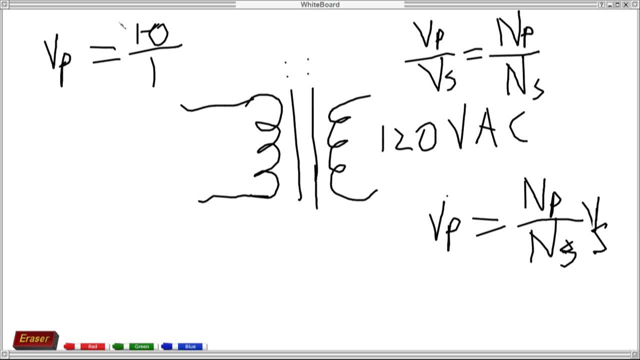 Okay, So um, what this means? it means that for every 10 turns on this side, which is, uh, which is your, um, your primary number of turns, there is 1 turn. So let's say you have 1000 turns here. 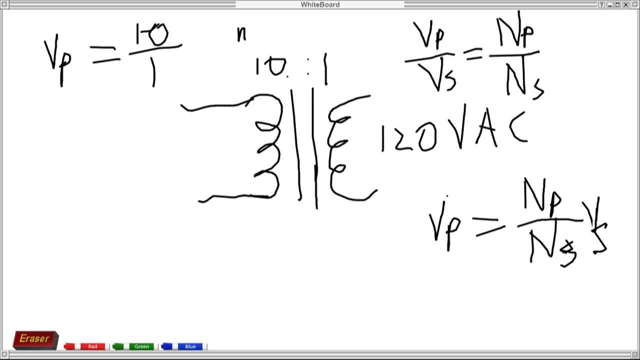 Okay, which is you know your little n. Uh, Let's say you have 1000 turns. okay, that means that all your sick on your, your secondary, you're going to have a hundred turns. so what this means is that? okay, I hope you got them. one dozen andсячons tournings per hundred. okay, let me leave. 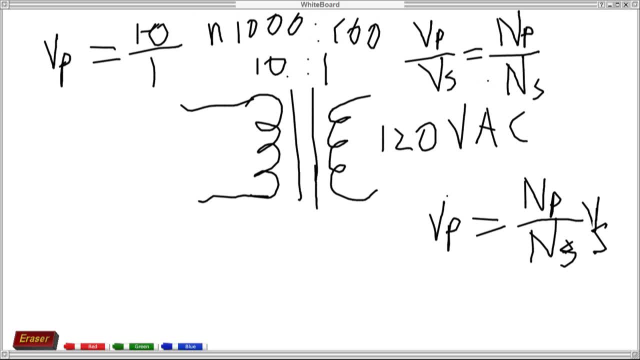 that there and remember: dismiss little. and this isn't the turn ratio. this is number of turns. no, not your turn ratio. okay, now let me erase this, and the ereye is gonna go by what she calls a full scale fill within a second and not. last thing you have to do is you have to put in your secondary voltage source. how? 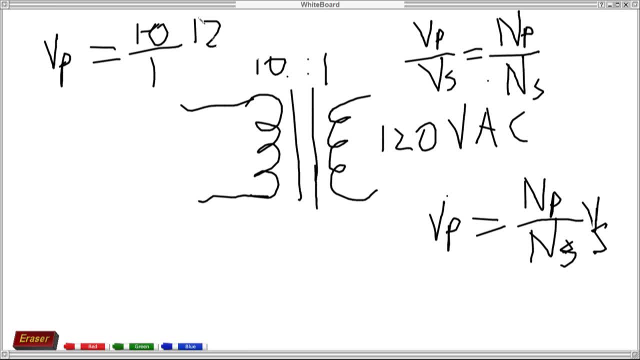 much you're getting from you, and we know it's 120, 120 volts AC. okay, so 120 volts AC times 10 is 1.2 kilobolts AC, or one dollar one thousand two hundred volts AC. okay, let me clean that up for it. it's a mess. so you have. 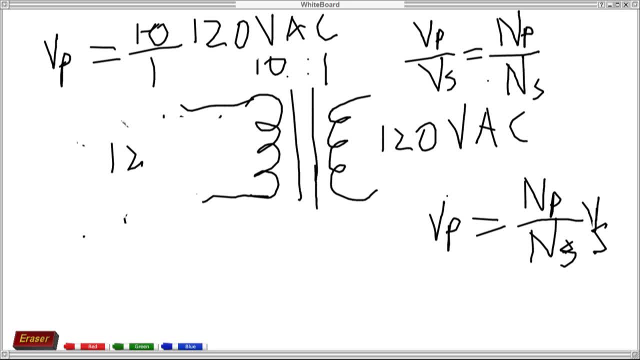 you have a, you have on this side one point: two kilobolts AC. okay, that's how much you need to feed in here, okay, and one thing: you have to keep in mind that the power, the power rating, the same amount of power you get you feed it, it's the same. amount of power you get. the same power you get on it. you power that 배reator. TAC power you get you feed. it is the same amount of power you get, at least, if not the lowest is basically the same amount of power. fun, you can get the same amount of power you get by. 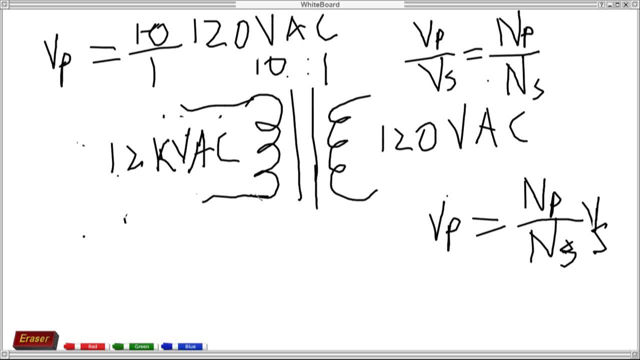 get at the other side, minus the magnetic, minus the power loss that you get to transference through the coils, the induction and so on. okay, so if you're curious how the how the transformers from the powers of power lines work, let me show you what in reality they do, at least for the residential grade. 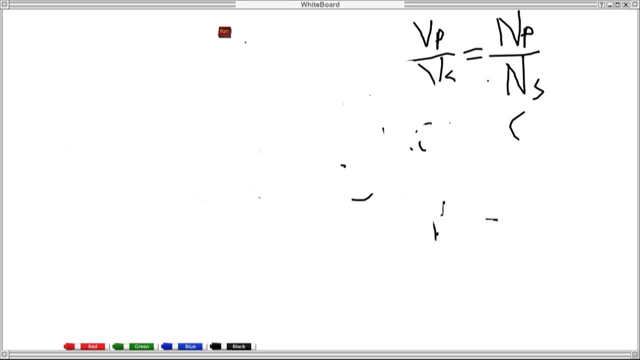 transformers. in reality is a little bit more complicated. okay, so basically, what they do is- this is so far from what I know- they get a 10 to 1 ratio. that's the ratio I just mentioned. it's a, it's isn't. I know it's an iron core. okay, you have. 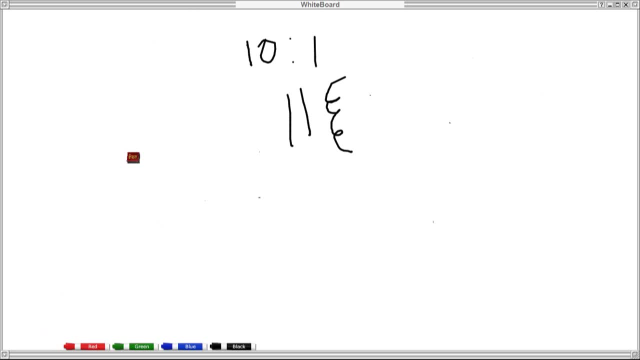 your. let me draw it better- okay, so this is the iron core, and right here you have your basic, primary, primary terms. okay, and this is 10. all right, this is a 10 ratio and this is a 1 ratio, but the thing is over here they do something a little bit different. 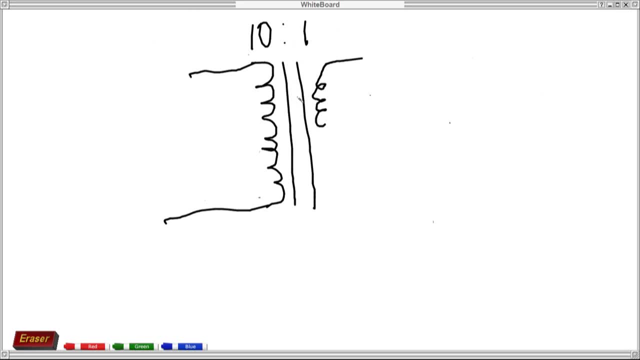 they do a number of turns and they do what they call a center tap, and a center tap is just pretty much a cut in between, an interruption in between the lengths of the coil. so this and the thing is that each one of these right here is 120 volts AC and over here is another 120 volts AC. okay, and that's. 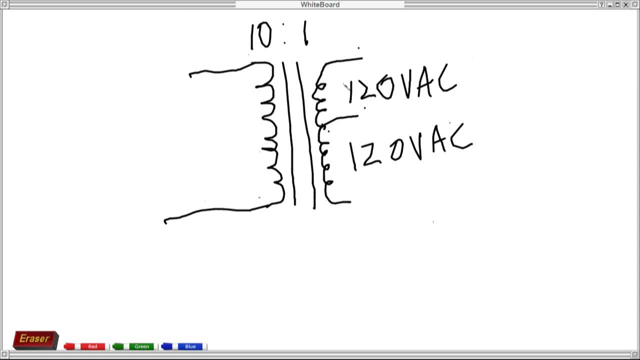 when you get from each point here, from here to here, 120 volts AC. that means from one ending to the center tap is 120 volts AC and from the center tap to here's 120 volts AC. okay. but however, if you get from this point here and this point here, okay, what you get is 200, 200, 240 volts AC. 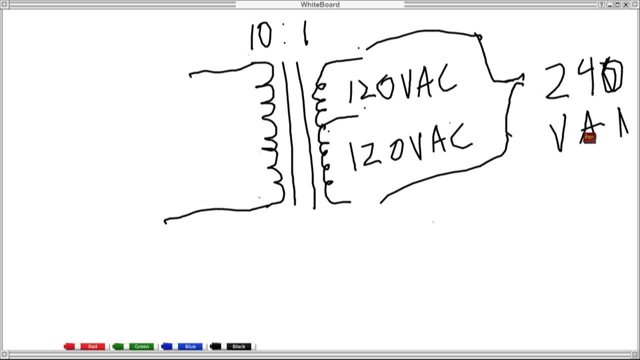 Okay, hold on, let me AC. okay, so you pretty much get that 240 volts AC from one ending to another, okay, and so that means that let's do our calculation here and what we did previously. and your, which is your B prime primary, which is here, which is equal to primary. 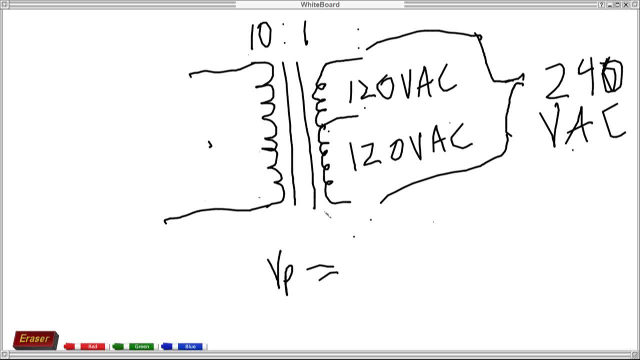 your primary turn ratio, which is 10, divided by 1,, which is your secondary turn ratio, times your, your secondary power source, which is 240,. okay, so you multiply that by 10 divided by 1, and what you end up getting here, right here- is you end up getting 2,. 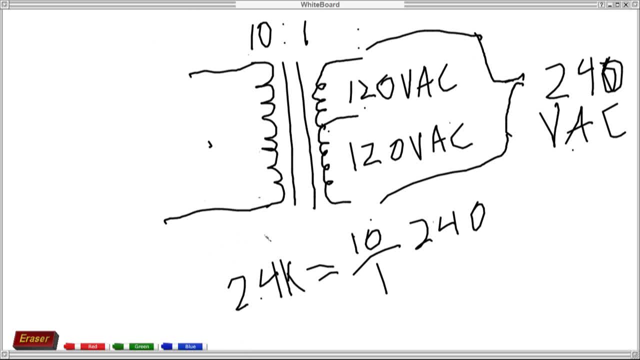 2.4 kilovolts AC. okay, so this is 2.4 K kilovolts AC, okay, and one thing, one thing that you have to keep in mind, is that one thing you have to keep in mind here. 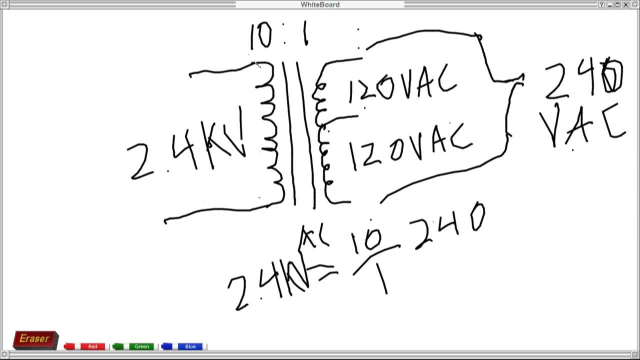 is that even though, because of this turn ratio, the, the voltage is the, the secondary voltage is divided by 10, the power main things the same. because even though the voltage, pretty much pretty much, is divided by 10, your current augments by that same number. 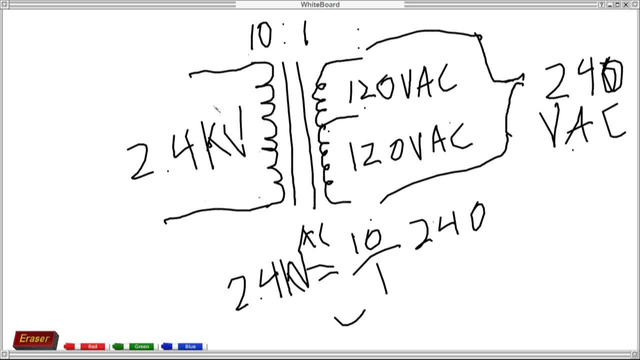 so if your feed- let's say you're, for example, You're feeding it- 1 ampere here, 1 ampere here of current Okay, What you would get on this end times 10, you would get 10 amperes. 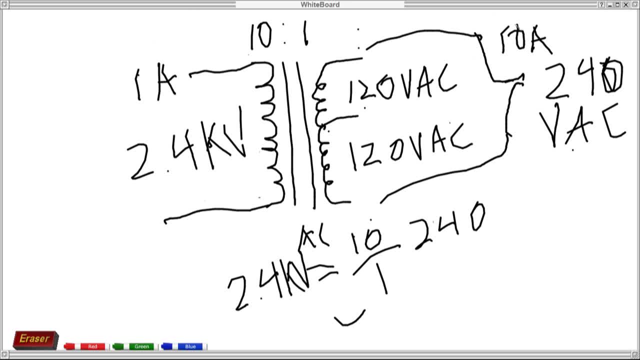 Okay, You'll get 10 amperes of current. Okay, So divided by here, since it's a center tap, that quantity would be divided in half, because instead you would get 10 amperes from 240 volts AC. 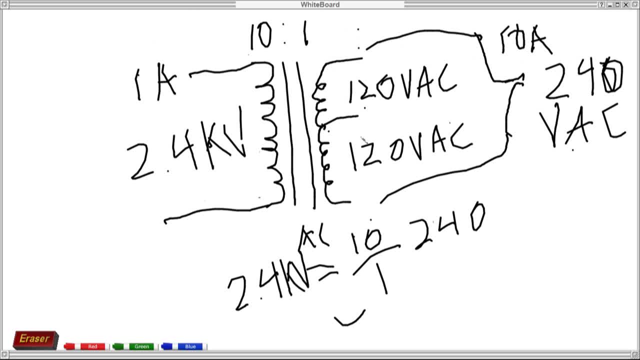 but if you get individually from here, you would get 5 from each, 5 amperes from each of the endings to the center taps. Okay, So this is basically the model, at least for the residential area on the power line transformers. 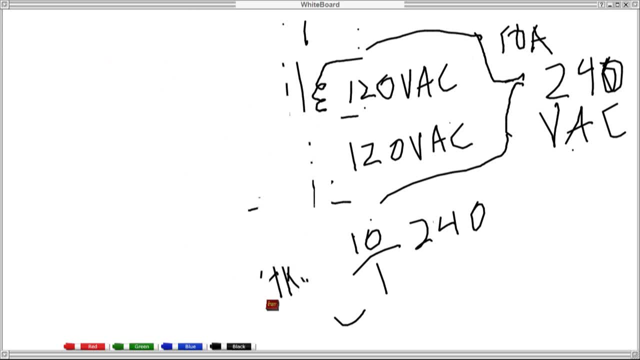 Okay, Now this is just one example of electromagnetic induction, but what they do in telecommunications it's a little bit different, because what they do is that it's basically it's basically the same deal. you're basically using a transformer. Now this is not including the whole antenna model and all. 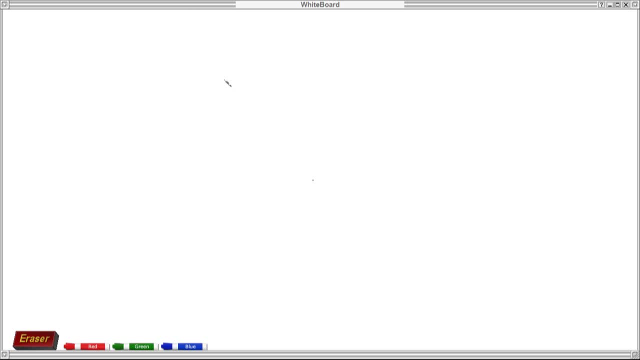 This is using, like, let's say, your Wi-Fi router or Bluetooth or your cell phone communication apparatus. Okay. So, just like you have a transformer here and you have your primary, you have your B primary, I primary, okay, your B secondary and your I secondary. 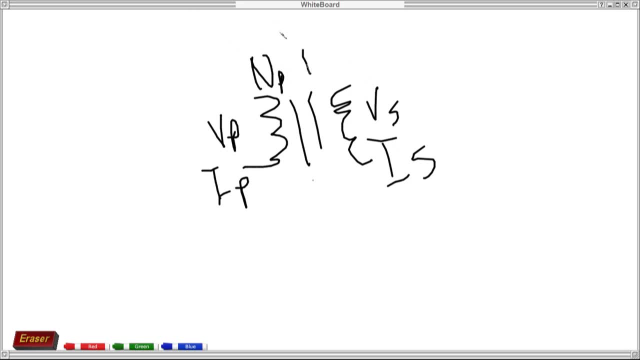 and then your turn: ratio: NP and S. Okay, it's the same, but the thing is that, instead of them using a complete iron cord which is connected to each other, what they do is this: they imagine each of these but separated, and what you have here is an air core, which is the distance, and they 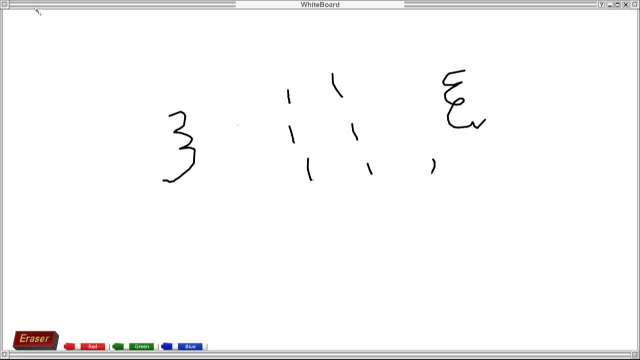 use a combination of different stuff on the inductors, and inductors isn't so really, and inductors is the apparatus in which you're inducing electromagnetic induction, and I'm gonna get to that a little bit further on, but that's pretty much the coils. it's inducing electromagnetic current from one. 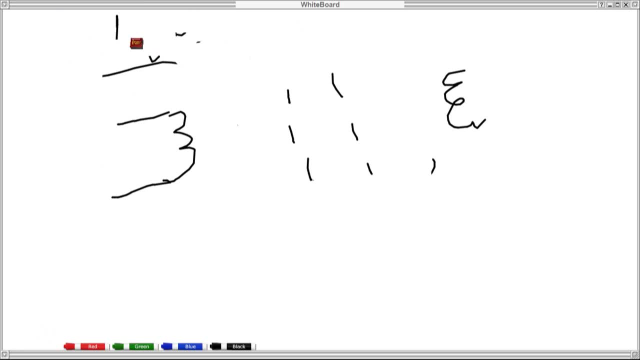 apparatus to another. okay now, so they use a lot of different stuff that they could use- iron or ferrite on each of the coils, and then there's the distance between them. okay, and keep in mind that that you, a lot of the time, you require substantial amount of power to. 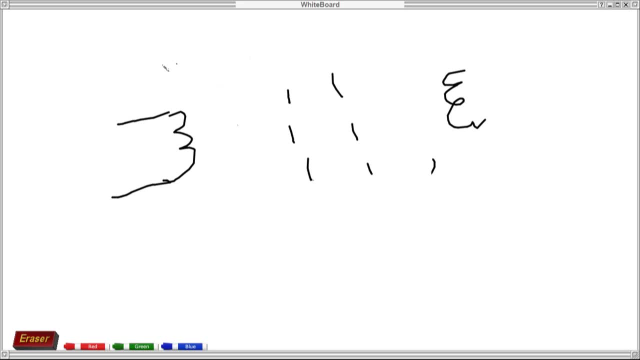 induce, depending on the range and all, and pretty much is it's just a separated transformer that that induces from one point to another. now, the drawback of this thing and is that it also induces current on other, on other other conductors that are around the area. that's your electromagnetic flux leak, because you, you're basically a 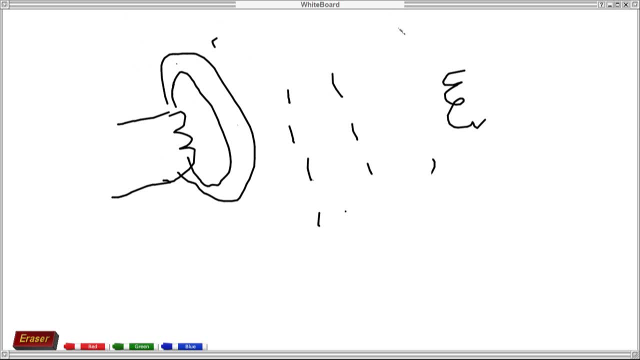 inducing current to to this apparatus here, and then current is being used here. so when do you, when you have a radio, when you have it one way where it induces and it receives? this is kind of like what they do on on an FM radio. okay, this is, of course, ignoring the whole deal of the, the and. 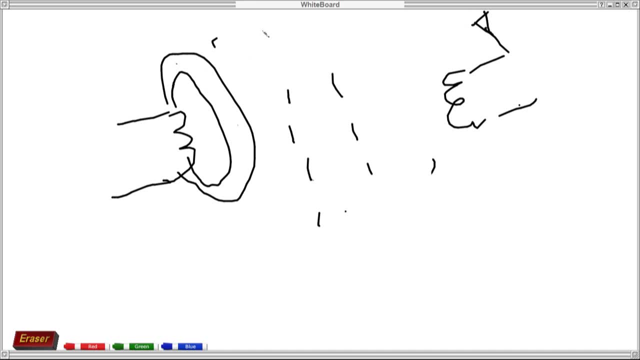 tenor that they put on here. but this is pretty much what they, what they do. okay, and it's induced one way. now, if you want to, now, if you want to have a like a back-and-forth communication, like two-way, you pretty much, pretty much what. 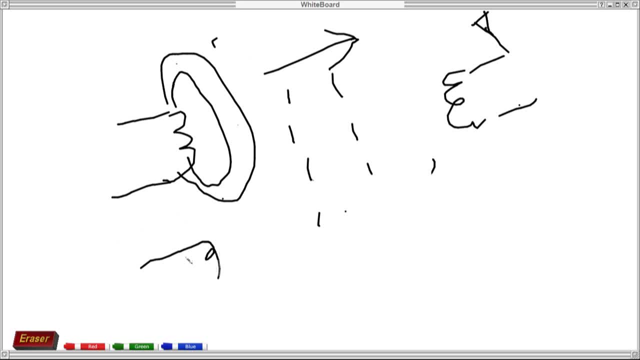 you need. is is kind of like a same coil also, but the deal is the deal is that this one is sending and this one is receiving, and this one is sending and this one is receiving. okay, and this is practically kind of like how Wi-Fi works, because you're sending. 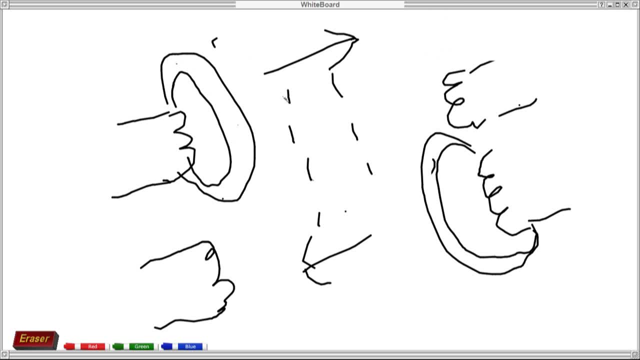 signals and you're sending signals to an electromagnetic field and you're sending and it's sending back. it's a transfer of data back and forth and if you ever notice your Wi-Fi router, you can see how many bits of transference back and forth and that's. that's where the whole deal with broadband comes in. 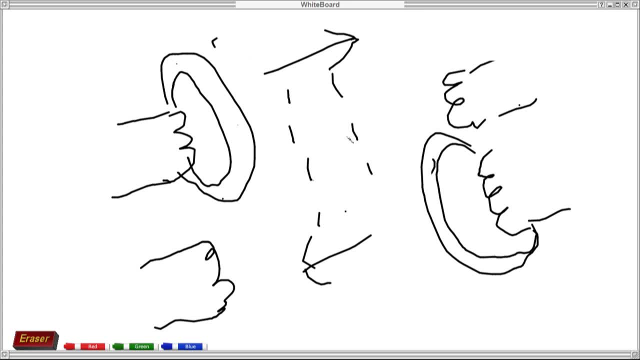 that, how much is your speed, your upload speed and download speed, and that's what applies here. okay, now the reason why I say ignoring the whole deal with with the whole deal with antennas, with the, with FM radios and all, is that pretty much I kind of messed up here. okay, okay, pretty. much kind of messed up here okay okay pretty much what what happened is that friend I got a new perceive whenever I get roughly 10 If you don't get that right you can get going vostro is gonna be potentially � job because I got a lot of entertainment going on it because As 다른anız que eu per reduzi em all aqui por a dar a number 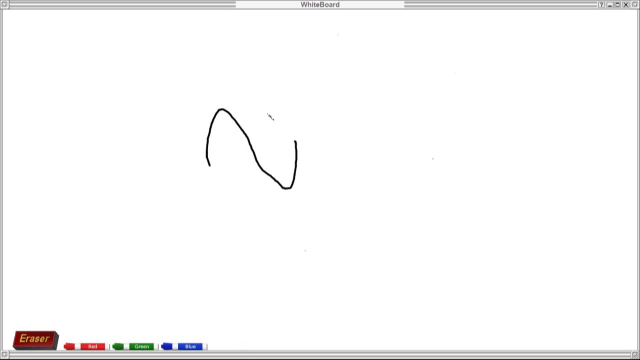 is that when you have a sine wave- okay- and I'm assuming you you have some knowledge into this- you have like a sine wave and this symbolizes the intensity of the magnetic field, okay, but at the same time you also have another. let me, let me draw this a little bit better, okay, 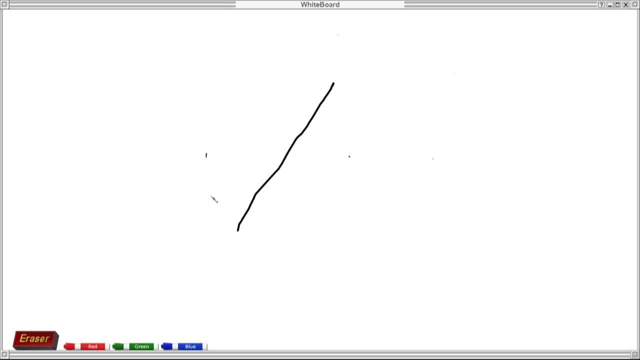 okay. okay, you have to sine wave here, okay, and you have like a little samplings here. okay, I'm not good at drawing, keep that in mind. but at the different aspects of the magnetic field you have a sine wave and you have like a little. okay, I'm not good at drawing, keep that in mind. but at the different aspects, 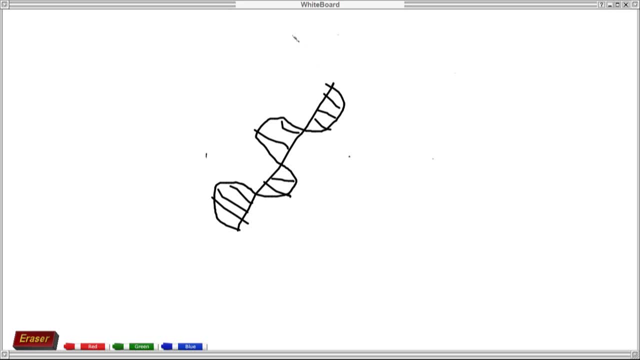 axis. let me draw the axis. this is like your premature y axis and this is your x axis, and then you have your, then you have your C axis. okay, you'll call this axis. this is like your previous axis is going to be like the sine wave, okay, and 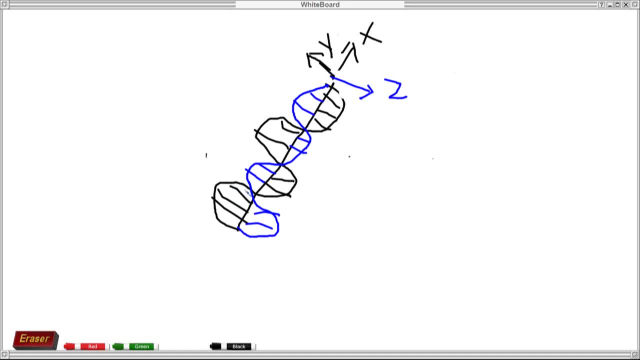 let's H or T easy, versus cosine G equivalent. so it's basically just a elliplical figure and then a sine wave- okay, and on that you have way, but also an ellipsoidal curve, okay, and if you move down the axis imagen, this the one thing. 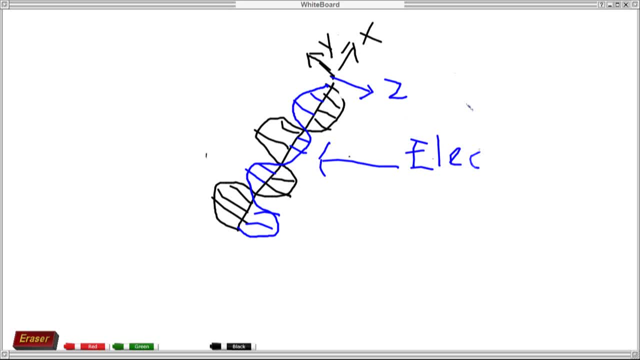 that I'm going to draw you just to let us know is: here is a flap beneath it. okay, maybe electric. this is your electric field and this one is your magnetic flux. okay, and one of the things that I forgot to mention earlier is this: let me kind of erase this and everything. 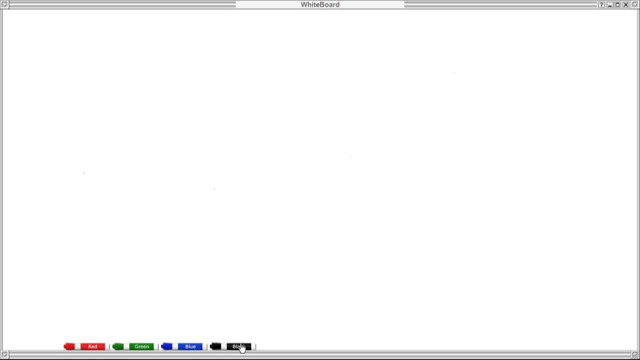 let's say you have an inductor. let's say this is a solid copper wire, okay. let's say this is a solid copper wire, okay. and let's say you have current flowing in this direction- okay, straight in this direction. okay, this current will have a magnetic field.